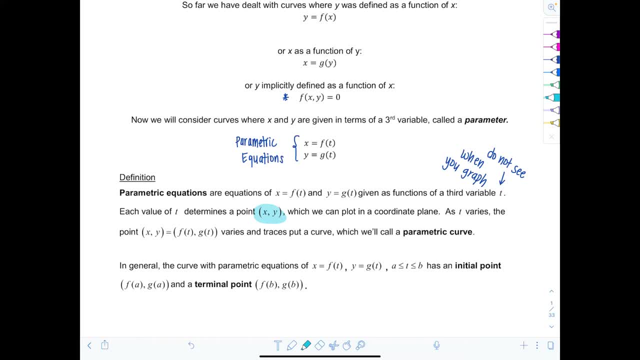 learned in the last few lessons. So we're going to have a very interesting graph here So we can plot in a coordinate plane And as t varies, the point xy, which we could write as f of t, g of t, that varies and it traces a curve which we'll call a parametric curve, Keep in mind for 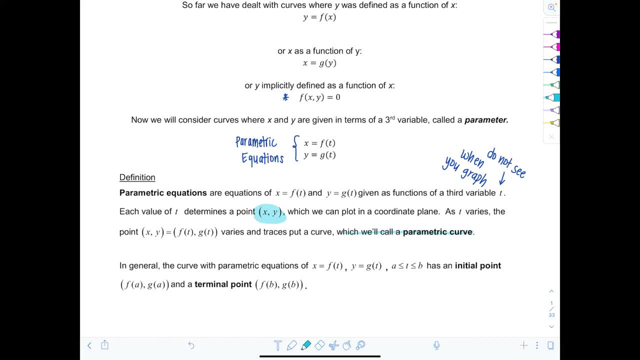 parametric equations, the direction of motion matters. So you're going to indicate that on all of our graphs And your, your parameter is always increasing, So you'll not have to worry. if you're worry, oh, what values shall I plug in for t to determine the direction of motion? t will always. 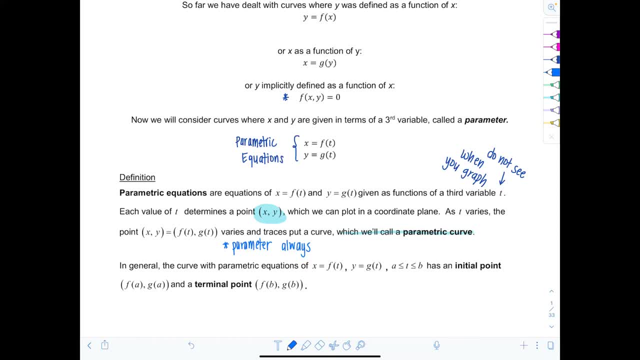 be increasing and as t increases then it traces out the curve. Okay, you could think of t. we didn't pick it arbitrarily a lot of the time it does represent time. So in general, the curve with parametric equations x equals f of t, y equals g of t and t between a and b has an initial point. 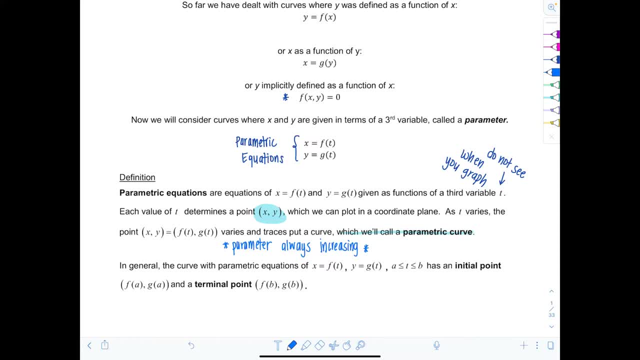 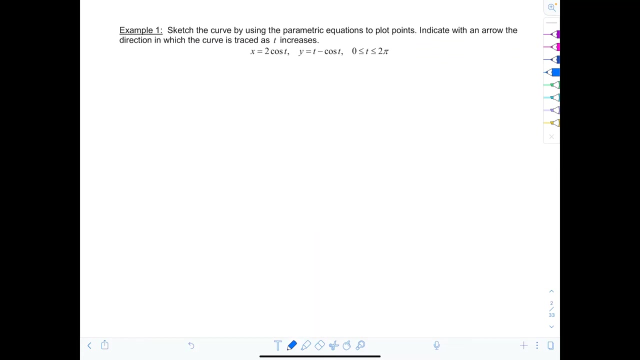 f of a, g of a and a terminal point. f of b, g of b. If no limits or bounds are given on the parameter t, then you can assume that it takes on any value within the domain of the parametric equations x and y. All right, so we will start off just nice and easy breezy and just plot some. 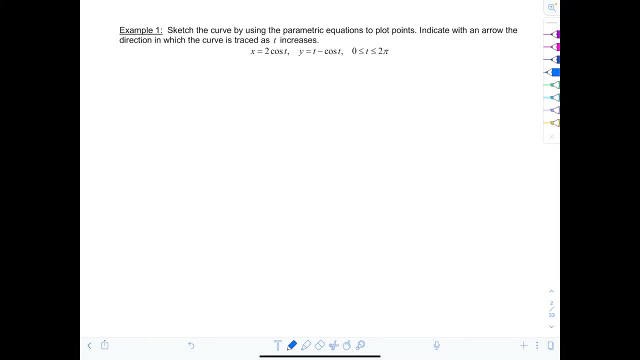 points and get a feel for what's going on. So example one: sketch the curve By using the parametric equations to plot points. indicate with an arrow the direction in which the curve is traced as t increases. So notice, in this case they are giving me limits on the parameter. 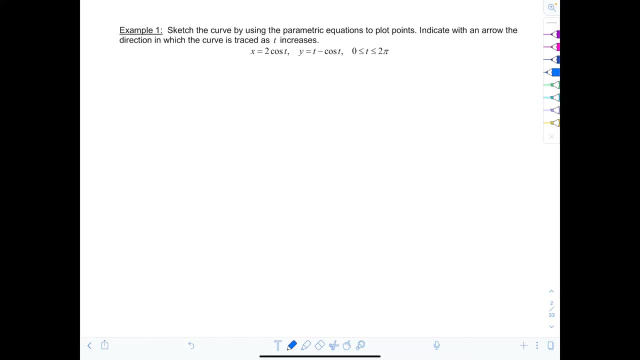 t is only varying between zero and pi. So I'm only going to plug in values between zero and two, pi inclusive for t, and then I'm going to figure out what the x and y values are by using the equations given. So x equals two cosine t, y equals. 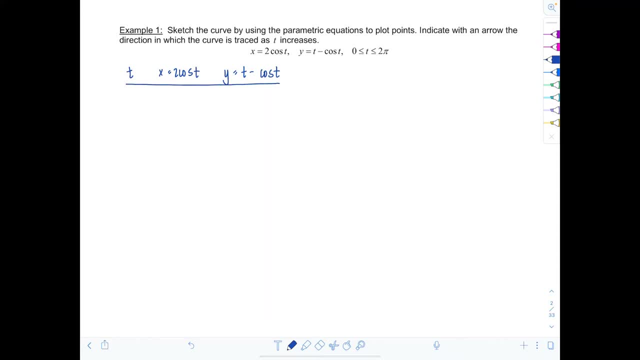 t minus cosine t, and then it's up to us exactly how many values we want to plug in, just enough to get a nice graph. When- and I'll show you later on once- we can kind of recognize what the graph's going to look like, then you may not need to substitute in so many. 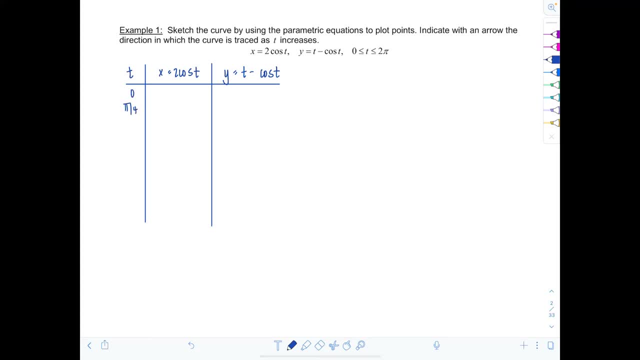 So I did quite a few. I did zero pi over four pi over two, three pi over four pi. So I just did increments of pi over two, three pi over four pi. So I just did increments of pi over two, three pi over four pi. 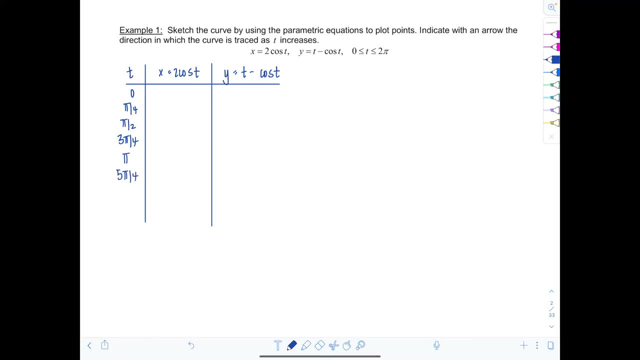 Then we have five pi over four, three pi over two, seven pi over four and two pi. And then from here you can just plug this in your calculator- Make sure you're in radian mode- And I have the following. You can just confirm: okay, So two, obviously two times cosine of pi. 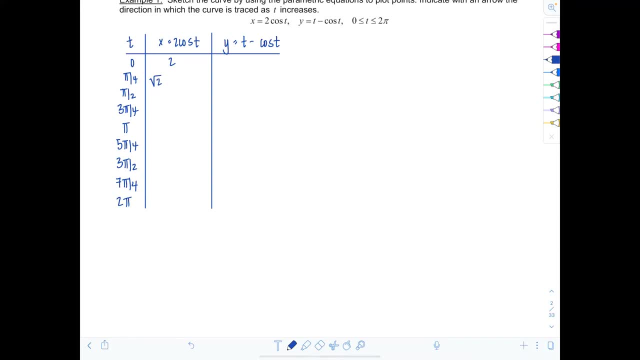 over four, that's rad two over two. So if I plug this in, I can just confirm: okay, So two, obviously, two times cosine of pi over four, that's rad two over two. So if I multiply by two then it's just rad two, which is about 1.4.. This is zero. 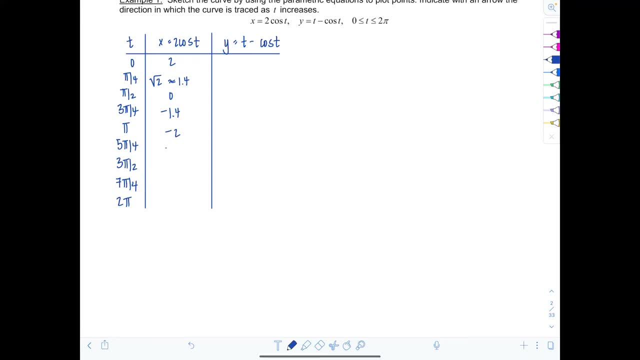 negative 1.4, negative two, same thing here: zero 1.4, and two. And then to get the y values, now you're going to substitute in the values of t into the equation t minus cosine of t. 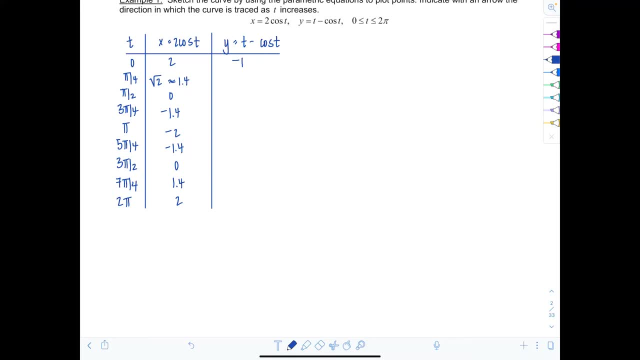 And just confirm. you should get the following negative one: 0.078.. I mean, honestly, that's a lot of decimal places. No one's going to notice if you plotted 0.078 or 0.08.. So you don't need. 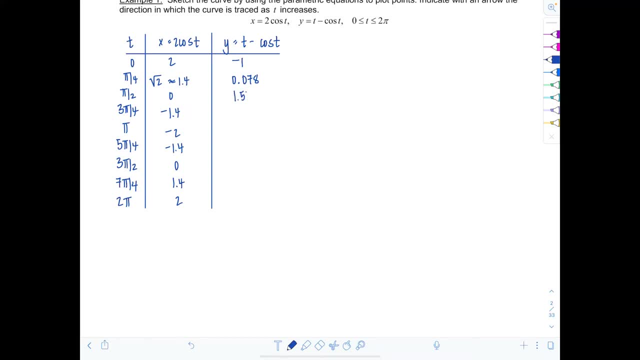 to go too overboard with the decimals here: 1.57,, 3.06,, 4.14,, 4.63,, 4.71,, 4.79, and 5.28,. okay, So here's how it works. if you've never seen parametric equations before, 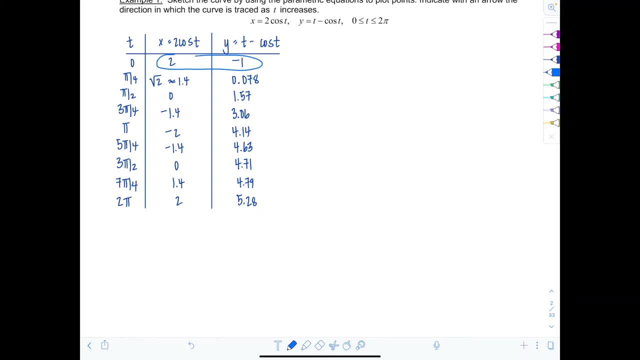 This right here is our first ordered pair. That's actually going to be the initial point on our graph. So 2, negative 1, that's our initial point. And then here's our next ordered pair: 1.4, 0.08, so on and so forth: 0, 1.57.. I don't normally list. 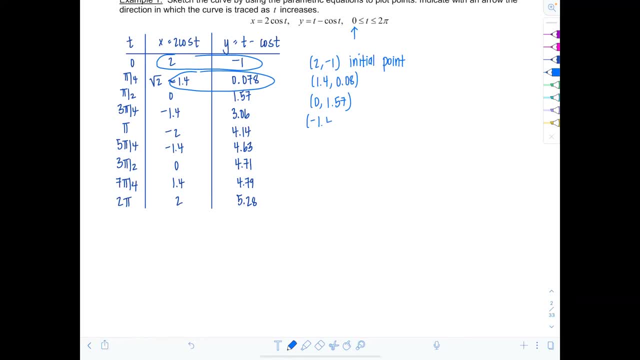 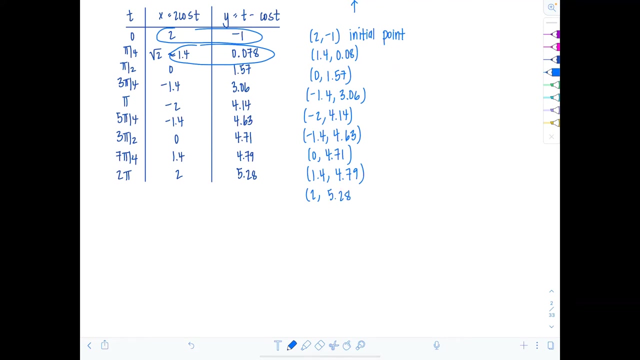 them out, but I will. It'll just make it easier to graph And in case you've never seen these before, I think it'll help. 3.06, negative 2, 4.14, negative, 1.4, 4.63, 0, 4.71, 1.4, 4.79, and then 2, 5.28.. And then this: 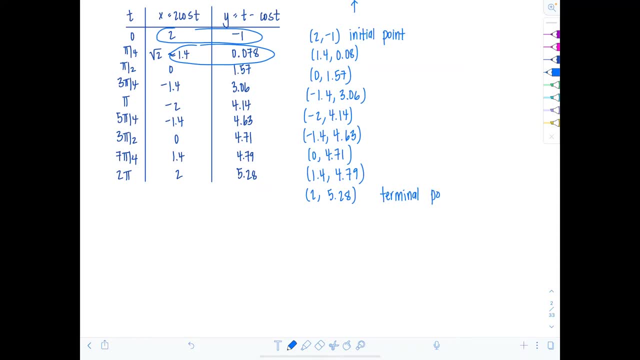 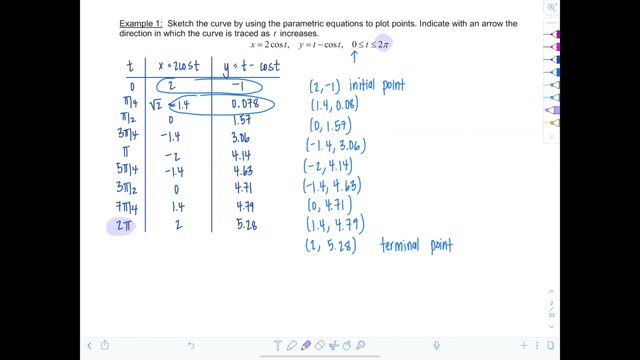 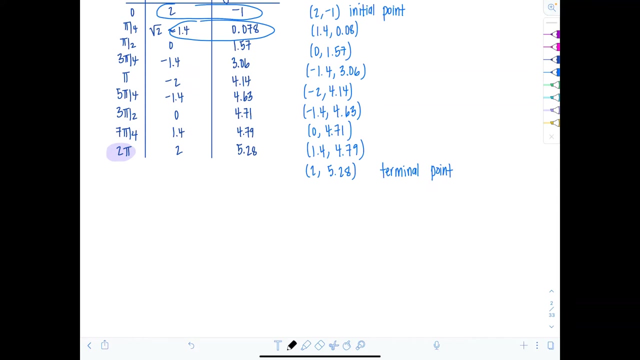 is our terminal point, Because notice that last point came from substituting in 2 pi for t, and that's what the end of the upper limit is on our parameter, the bound. okay, So now let's plot it. It looks like in the x direction. we just live between 2 and negative. 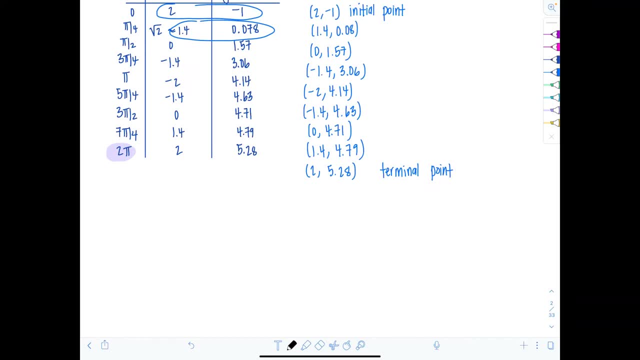 2. And then, in the y direction, we go down to negative 1, but I have to go up to a little more than 5, okay, So let's do it, And let me scoot this over. I just had an idea. 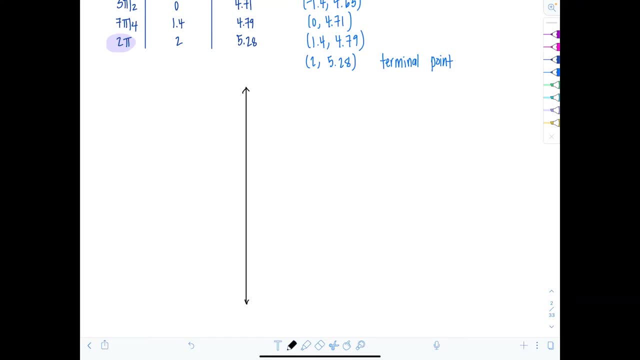 So not too much negative. y right, we said that. Okay, so here's the x-axis, y-axis, it's gonna go up to 6, 1,, 2, 3, 4, 5, 6,. love it. 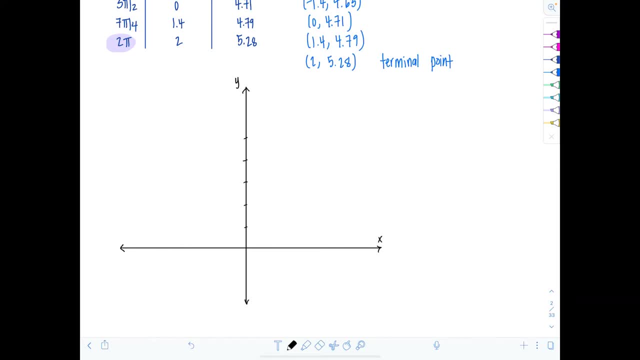 Let's compute So: 1.2, 4.27.. 1.2, 4.28.. 1.2, 3.23.. it Looking good? Does your graph look nice? Take pride, Be a strong grapher, It'll set. 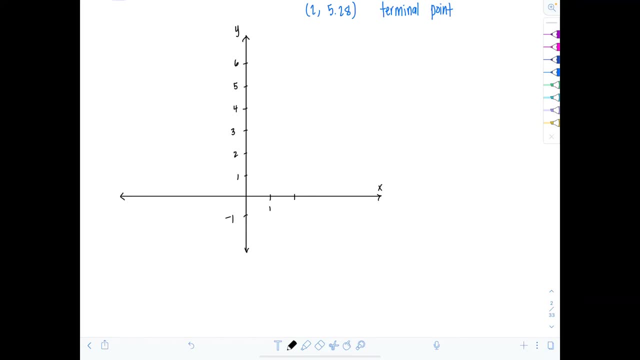 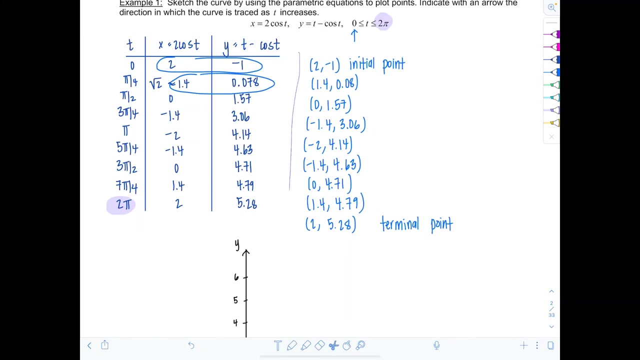 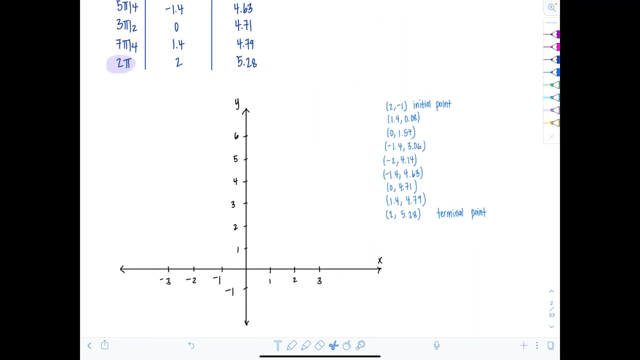 you apart. Negative one, and then one, two, three. Let's go the other way. Okay, Looking good. Then I have this bright idea. Let me put this right next to the graph so I don't have to keep scrolling. Shrink it down, Perfect, Okay. So here we go. Two, negative one, That's. 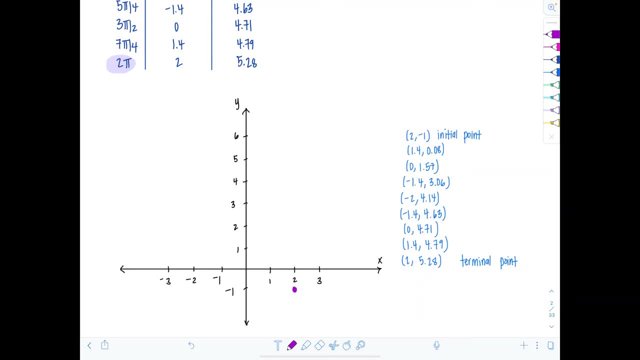 my initial point, And sometimes I do like to indicate: hey, guess what This comes from? substituting in t equals zero, Then we have 1.4.08.. Okay, So 1.4, and then just barely, barely above the x-axis, Love it. 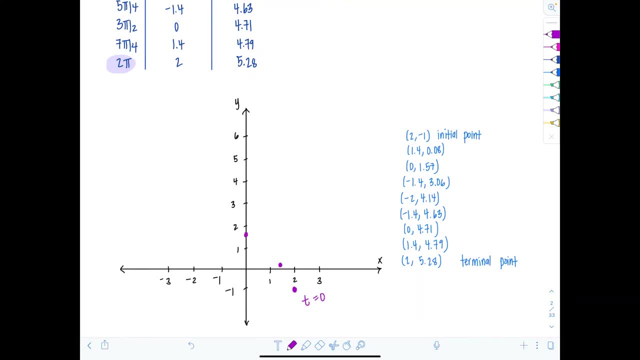 0, 1.57.. That looks like it's there. Negative 1.4, 3.06.. Maybe around here Negative 2, 4.14.. So four and a wee bit more. And then, oh, look at what's going on here- That it's. 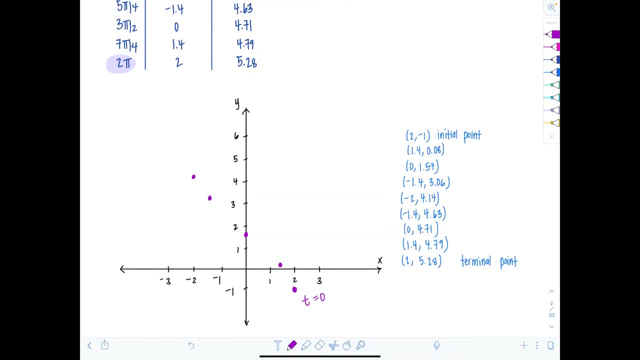 turning back around: Negative: 1.4, 4.63.. Okay, Let's trace out what we have so far. It's going, it's going, it's going. Changes its mind And we can put these little arrows here to indicate the direction of motion. 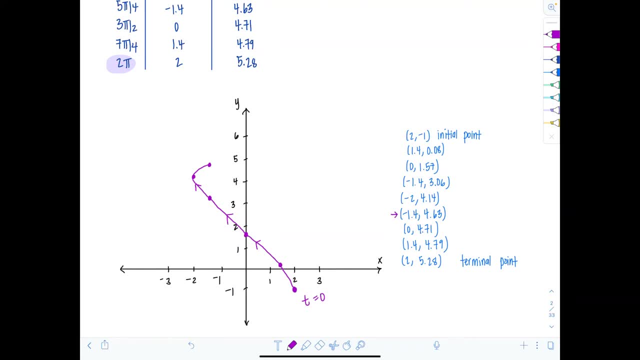 Let's see, I stopped here. Negative 1.4, 4.63.. Then we've got zero 4.71.. Okay, 1.4, 4.79.. So it's just barely coming up here. And then two 5.28.. So maybe here, And that's the terminal. 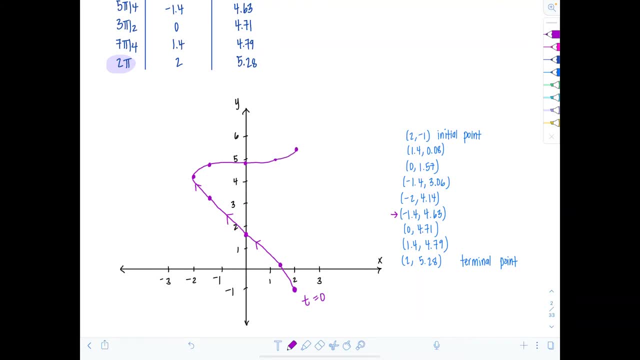 point. Okay, So it's just barely coming up here, And then two 5.28.. So maybe here- And that's the terminal point This comes from- t equals 2 pi. All right, Make sure when you're given limits on your 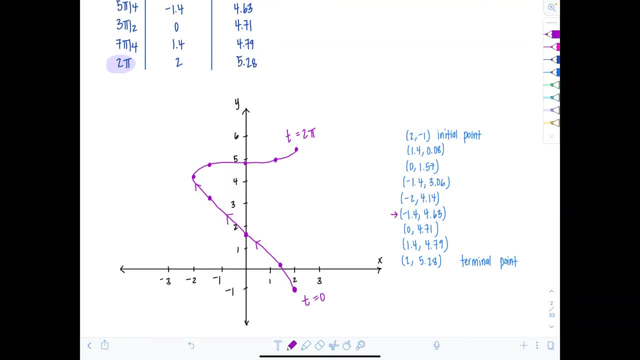 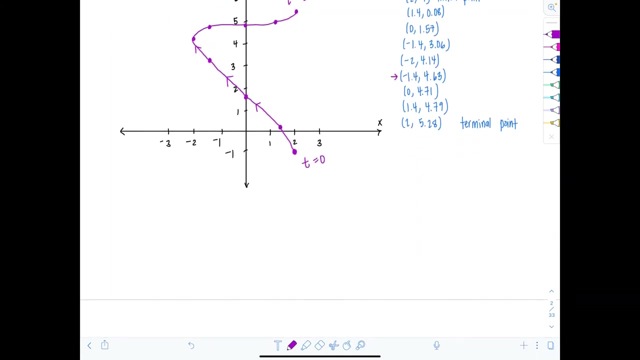 parameter that you clearly showed the initial and terminal points. If there's no limits on the parameter, then make sure you indicate that you have arrows when appropriate. All right, So that's that first example. How was it? Very good. Let's move on and look at something. 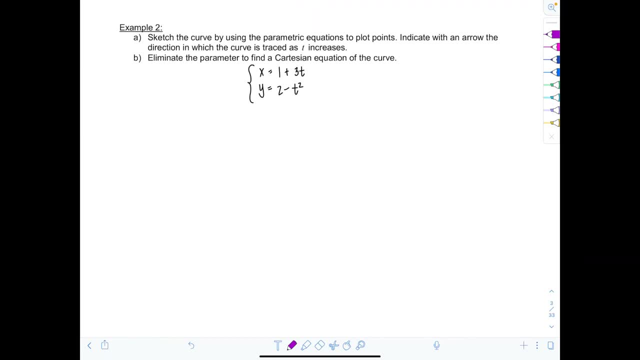 else. So this is part H, So this is part k. All right, Here's a little看到. If we've left out part e, we're going to use. par is equal to part b. that the平 director goes to t. Then put the numerical and the statement as an answer for it. 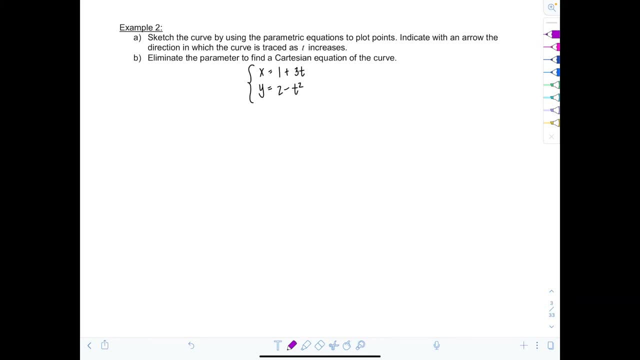 All right. Example 2 says: sketch the curve by using the parametric equations to plot points. Indicate with an arrow the direction in which the curve is traced as t increases, And then, part b, eliminate the parameter to find a Cartesian equation of the curve. So 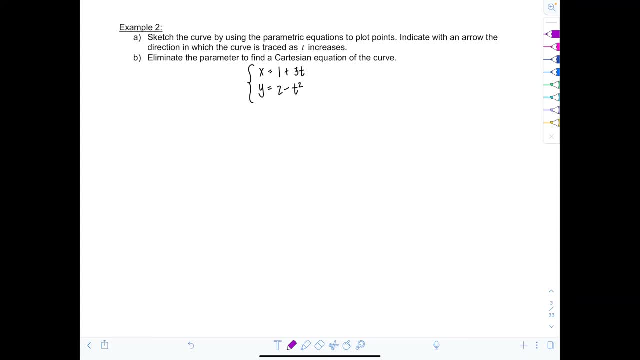 if you'll notice, here with these parametric equations there's no limits given on the parameter t And I notice that for both equations x and y I can substitute in any value x, the Y coordinates. We don't know the parameters, We only use parameters such as pi and q and s, which is right here. 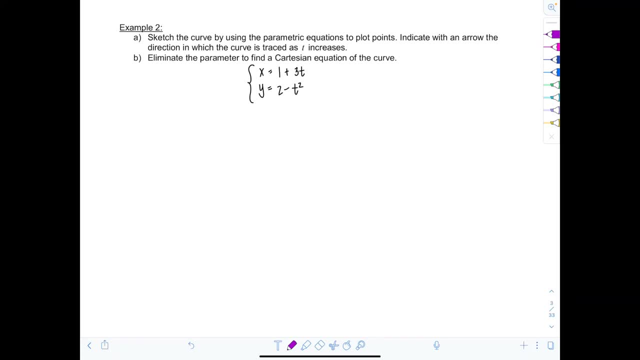 in any value of t, and they will both be well defined. So it's up to you- kind of use your judgment- what you want to start off with. I'm going to go from like negative 3 to positive 3 for my parameter t, see what sort of values I get for x and y, and then I'll determine from there. 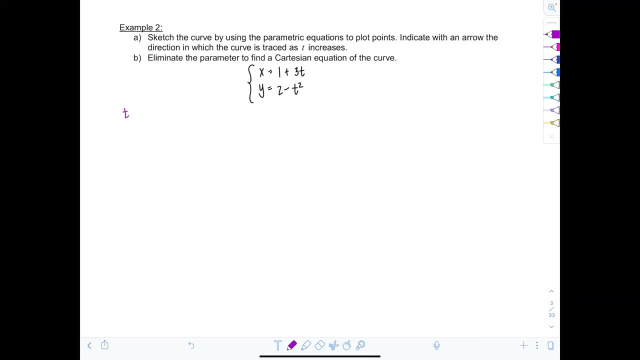 if I feel like I need to plot more. Okay, so here's t, x, y, and so we'll start from negative 3,, go to positive 3, that should give us like a nice starting off point. So negative 3, negative 2, negative 1,, 0,, 1,, 2, and 3.. And then we'll figure. 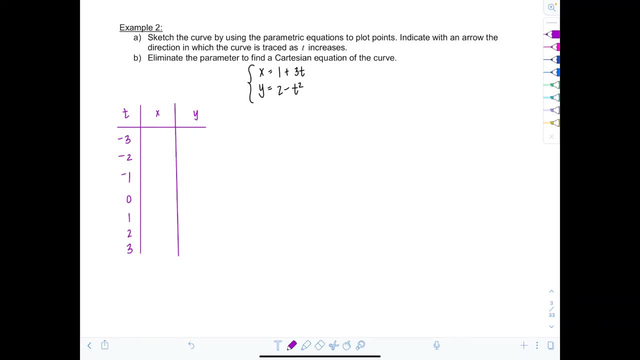 out what the x and y values are that correspond. So let's see if t is negative 3,- remember I'm substituting that into the equation right here. x equals 1 plus 3t, So I'd have 1 plus 3 times negative 3, so that's going to be negative 8.. If t is negative 2,: 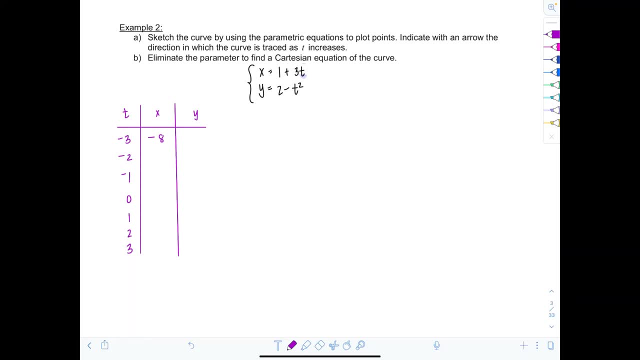 x is going to be, let's see 1 plus 3 times negative 2, so that'll be negative 5.. And then you notice that equation is linear, right? So all of these values just go up by 3,. 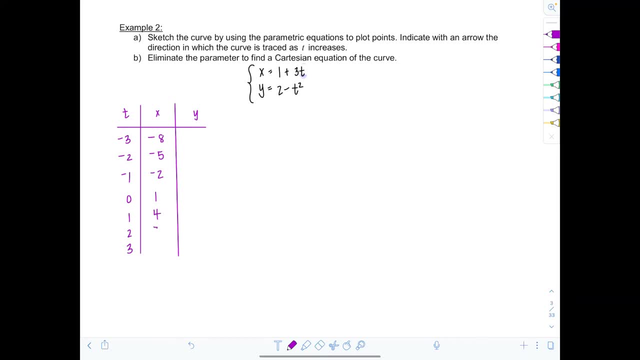 so I can just keep adding 3, call it a day, Okay, Beautiful. And then for y it's 2 minus t squared. so 2 minus now negative 3 squared, that's going to be positive 9, so this is negative 7.. 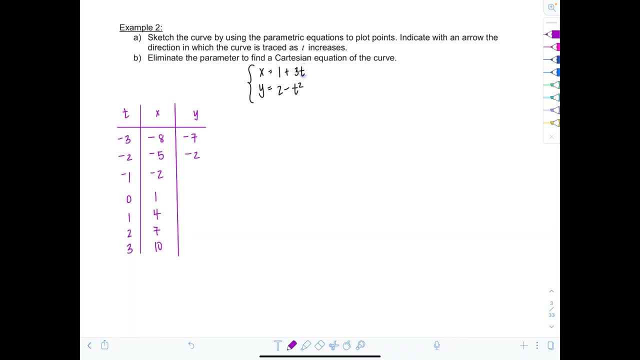 Then 2 minus 4, that's going to be negative 2, 2 minus 1,, 2 minus 0, and then they repeat: right, So 2 minus 1, then I get negative 2 again and negative 7.. All right, So let's see here: 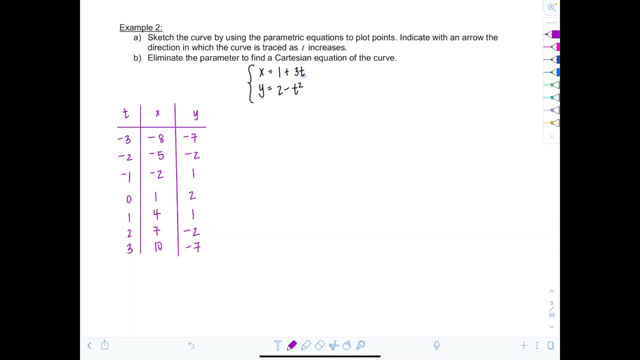 it looks like it's going to be negative 7, and then I get negative 2 again and negative 7.. So it looks like x values need to range between negative 8 and 10.. Okay, that's not bad. And then y values only go up to positive 2,, mostly in the negative. so I'll draw my axes accordingly. 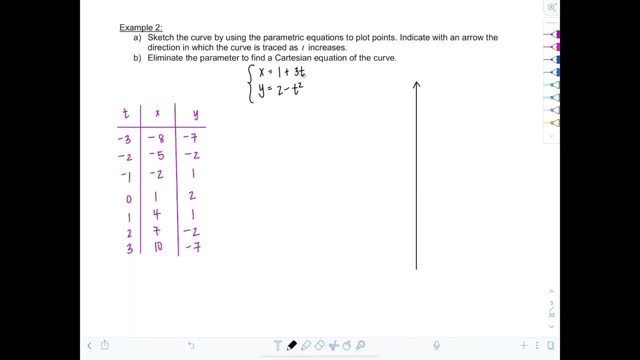 All right, Always look at what sort of points you're going to have to plot before you draw out your x and y axes, so you can do it in a way where you set up for a nice graph. So here's the x-axis, here's the y-axis. I have to go up to 2,. 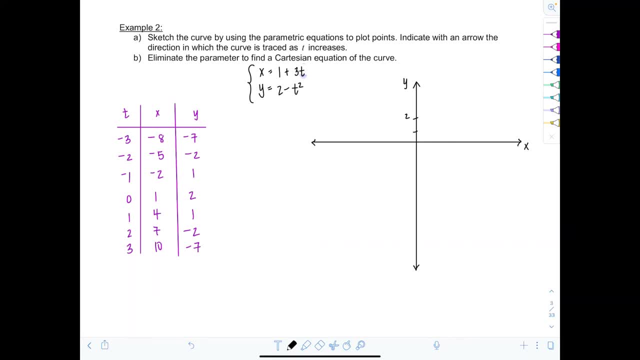 so 1,, 2, and down to negative 7.. So 1,, 2,, 3,, 4,, 5,, 6,, 7.. And then the x-axis has to go negative, 8 to positive 10.. Let's just scale this guy by 2.. So that's negative 2,, 4,, 6,. 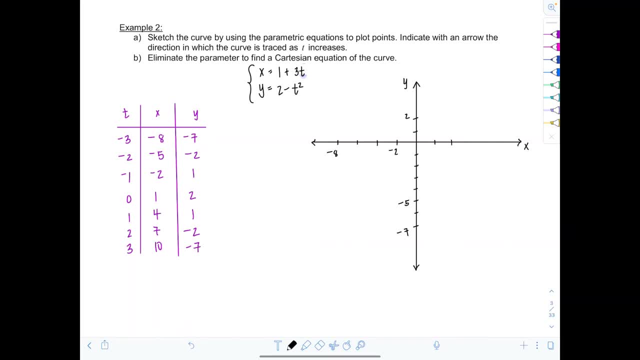 8, and then positive 2,, 4,, 6,, 8,, 10.. All right, You don't have to scale your axes. the same right, Just label and all is good. Here we go. I'm not going to list the points out, Hopefully, at. 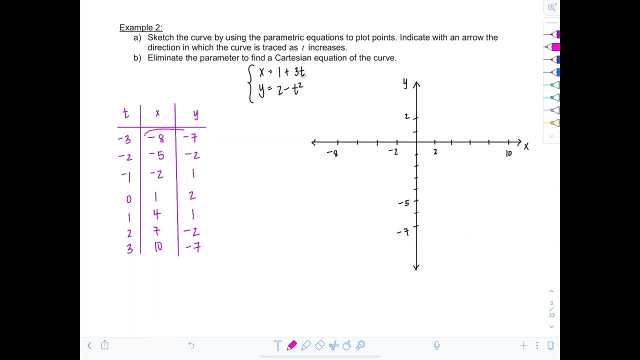 this phase in your math career, you know this is negative 8, negative 7.. Let's plot it, people. So negative 8, negative 7, right here. Then we've got negative 5, negative 2.. So that'll be about. 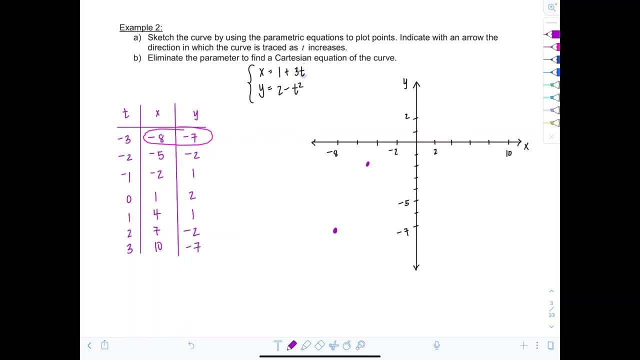 here, Remember, I'm scaling my axes differently: Negative 2, positive 1, then I have 1, 2. All right, Then 4, 1. Got it. 7, negative 2.. So 2,, 4,, 6,, 7,. 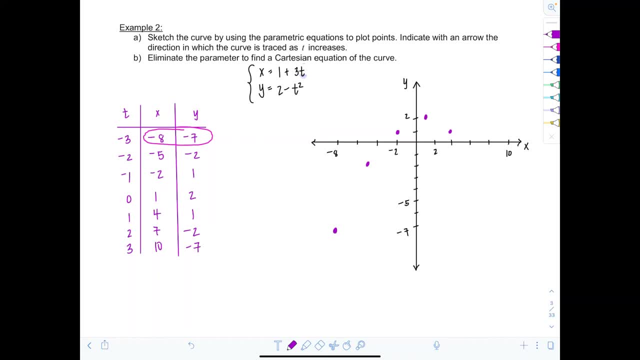 and negative 2 would be here, And then we've got 10 and negative 7.. All right, So in this case I'm still going to indicate the direction of motion. All right? Okay, It went down this way. I know it keeps going, So put an arrow on that end of the graph. 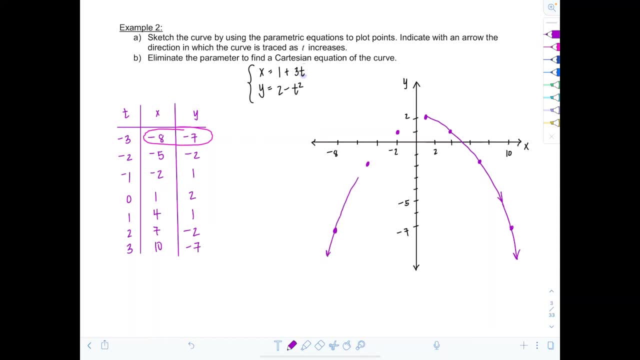 And same thing here. It keeps going down that way. That's not for the direction of motion. That's to indicate that the graph keeps going. This little arrow here is for the direction of motion. Okay, So as t increases, we went up one side of the graph, back down the other side. 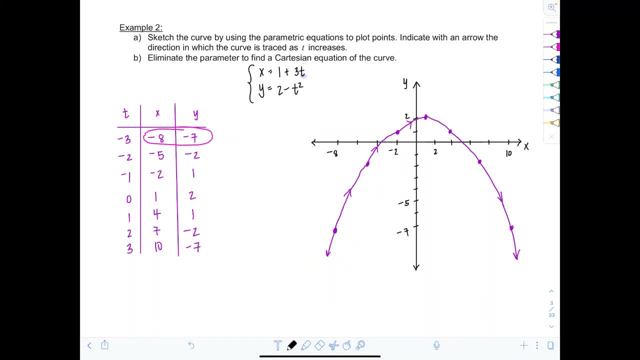 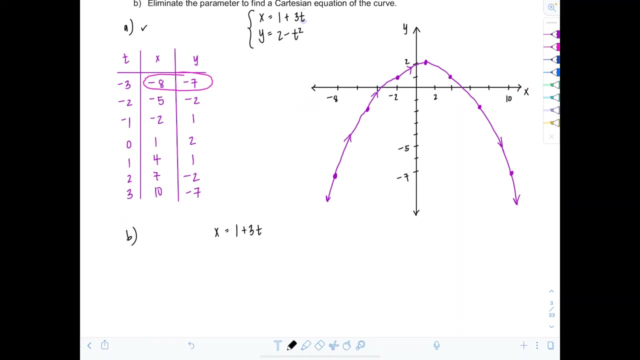 Very lovely. That's part 2.. Part A all done, Okay, Check. Part B says: eliminate the parameter to find a Cartesian equation of the curve. So let me rewrite the equations here and I'll show you exactly how we do that. So we have x equals 1 plus 3t and y equals 2 minus t squared. There's a few little. 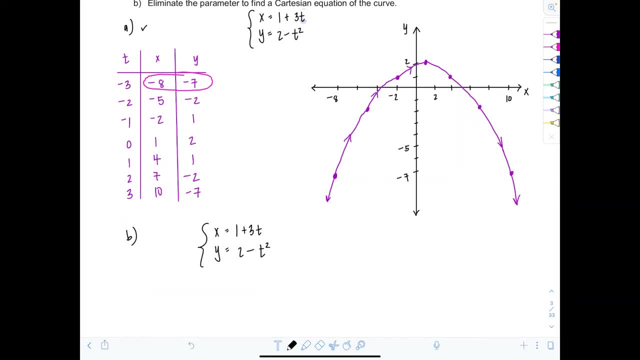 techniques that you can use to eliminate the parameter. One of the most useful is just substitution. So solve for the parameter in one of the equations and then we're going to do the substitution. So solve for the parameter in one of the equations and then we're going to do the. 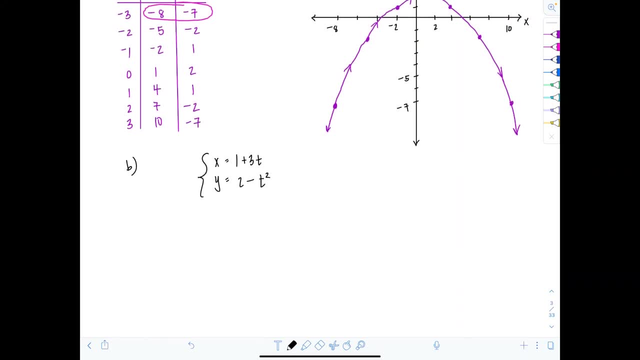 2, and then substitute it into the other equation. Since it's going to be easier to solve for t in the first equation, right, since t isn't squared, I'll go ahead and do that and then substitute it into the second equation. So solving for t- I have x minus 1 over 3- is equal to t. 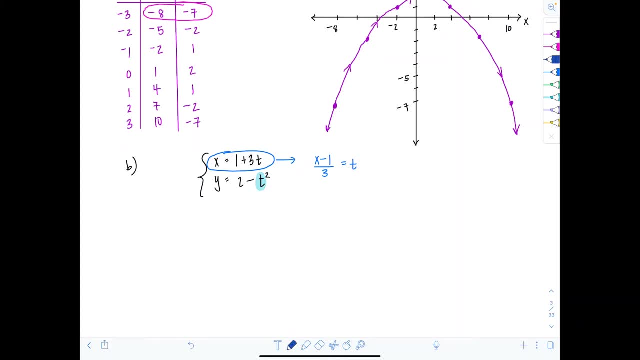 and then now let's substitute that in below, So then we have y equals 2 minus instead of t. I'm going to put x minus 1 over 3. 3 squared. And then let's simplify this a little bit. I mean, I can already tell this is going to. 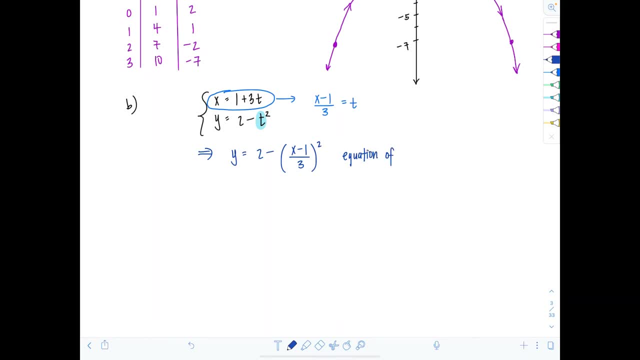 be the equation of a parabola. How do I know? Because I have y solved in terms of x and x is squared And we just reviewed parabolas. If you want to rewrite this in vertex form, you can go ahead. notice: this is going to give me a coefficient of 1- 9th, And I still have that negative there. So 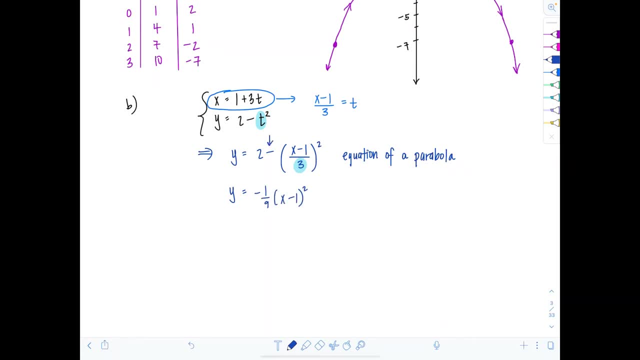 that would be negative 1, 9th times x minus 1 squared plus 2.. And if you'll remember, when we have the vertex form of a parabola, it's written as: y equals a times x minus h squared plus k. 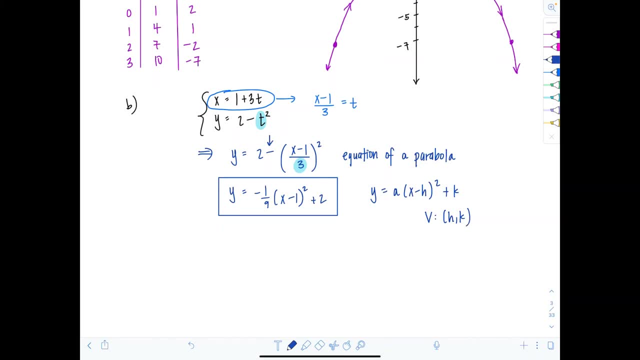 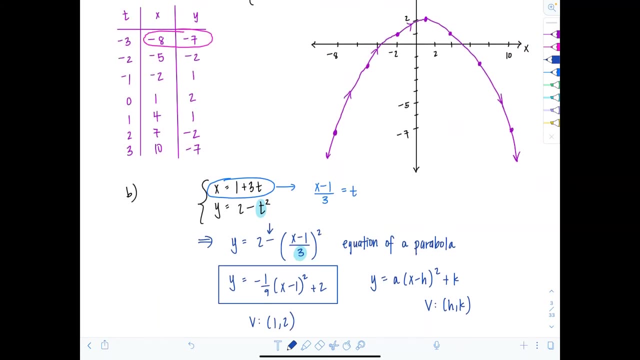 where the vertex is at h comma k, And, And. so here I can tell: okay, the vertex of this parabola is at 1, 2.. And indeed that's what we found when we graphed right. Oh look, there's our vertex. 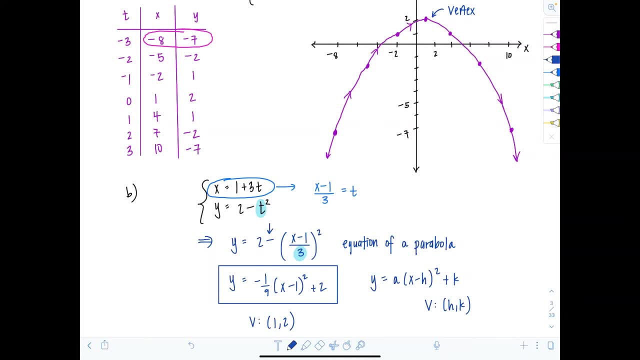 Beautiful, Okay. so, as you can see, it's very useful sometimes to eliminate the parameter so you can identify what sort of curve you're dealing with, And that can make it more straightforward when it comes to graphing, So you're not just plotting points without a clue as to how things are going to turn out. 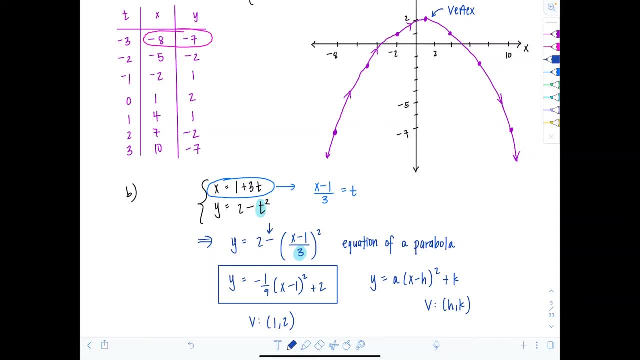 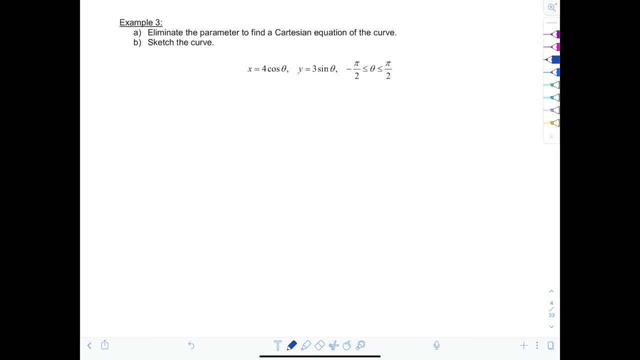 But when you already know what sort of curve to expect, life can be easier. So let's practice doing that some more. So example three: eliminate the parameter to find a Cartesian equation of the curve and sketch the curve. Now this little scenario comes up so much. 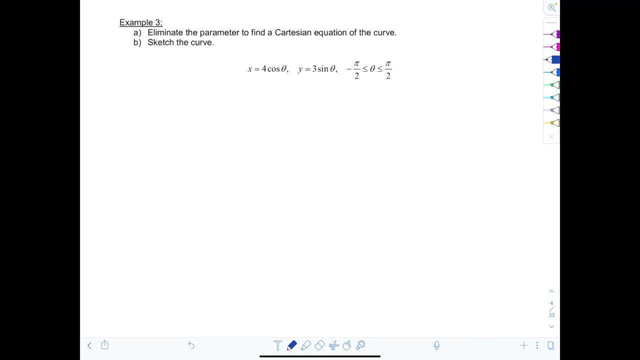 So I wanted to show you the technique. We have: x equals 4 cosine theta and y equals 3 sine theta. Now, anytime you're working with trigonometric functions, a lot of the times- one equation will be given in terms of the number of times you're working with trigonometric functions. 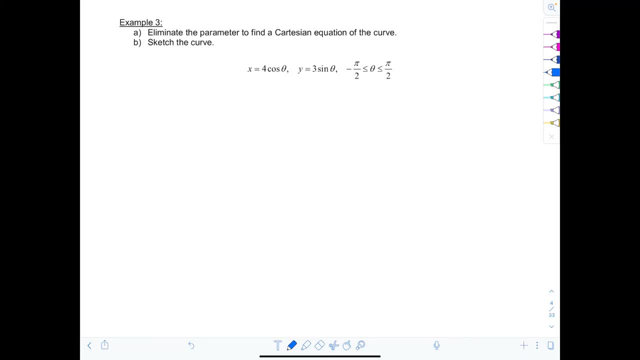 In terms of cosine, the other one's sine, Or you might see like a tangent and secant, And the reason is because you're going to use a Pythagorean identity to eliminate the parameter Watch. So we're going to use sine squared theta plus cosine squared theta equals 1. 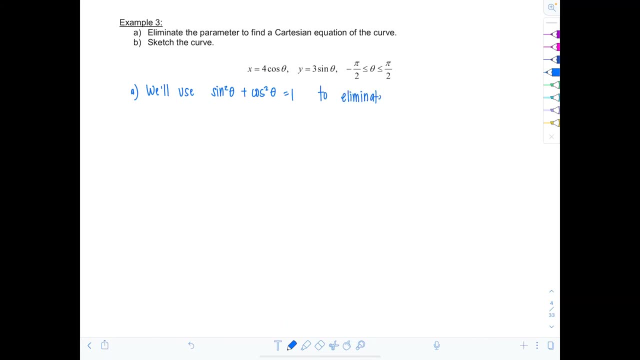 to eliminate the parameter. You will wow your friends when you do this. So we know. they told us x equals 4 cosine theta. That means x divided by 4 is equal to cosine theta, correct? So then I can say: all right, x over 4 squared is equal to cosine squared theta. 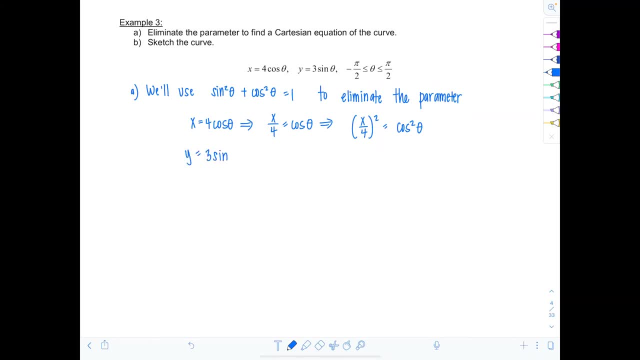 Similarly, since y is equal to 3 sine theta, that means y over 3 equals sine theta, which means y over 3 squared, That means y over 3 squared is equal to sine squared theta. And then, if I go ahead and add these together, 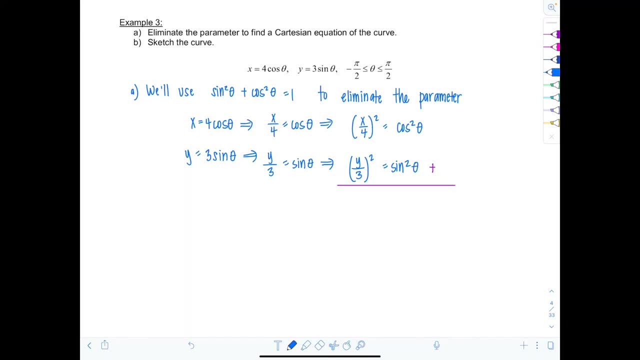 now I'm adding cosine squared theta and sine squared theta, And what do I end up with? x over 4 squared plus y over 3 squared equals 1.. So there, I've eliminated the parameter Beautiful. Now part B asks us to sketch the curve. 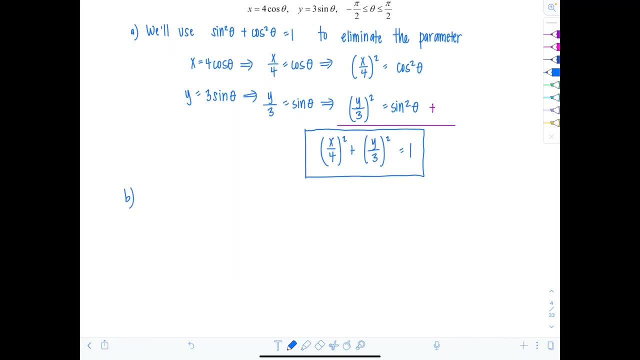 Okay, no problem. Do you recognize this equation? Hopefully you do, because you've just reviewed your conic sections, or you will shortly, but you should have seen them in pre-calc, at least a little bit. So this is the equation of an ellipse centered at the origin, right? 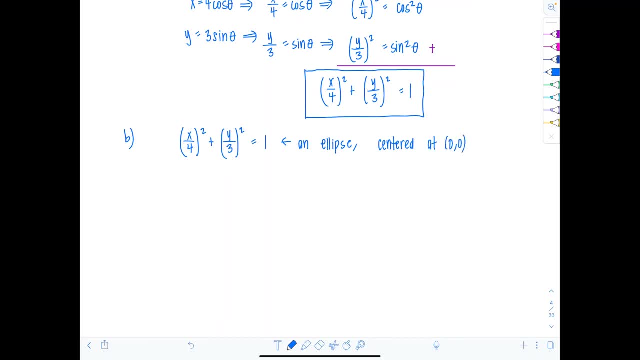 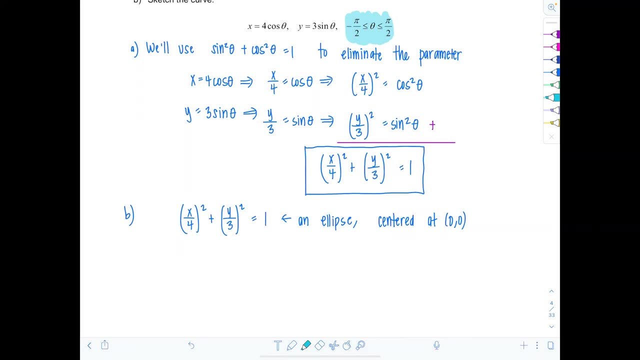 So just centered at 0, 0.. And notice, they gave me a restriction on the parameter. In this case the parameter was theta, not t, no big deal. And theta is restricted between negative pi over 2 and pi over 2.. 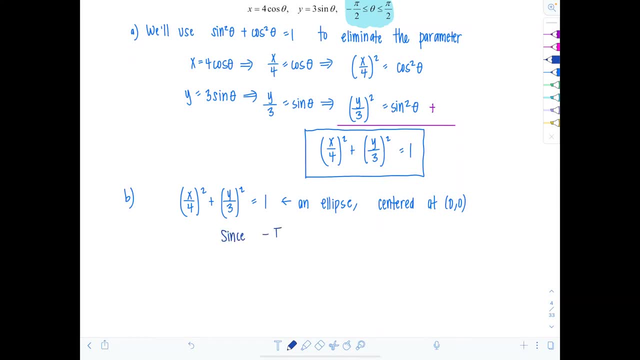 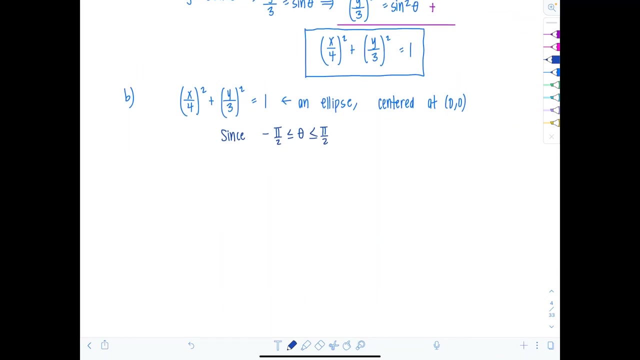 Well, what does that mean? Okay, well, since theta is restricted between negative pi over 2 and pi over 2, I'm only going to trace out part of the ellipse. Can you figure out which part? Well, plug in each of the values. 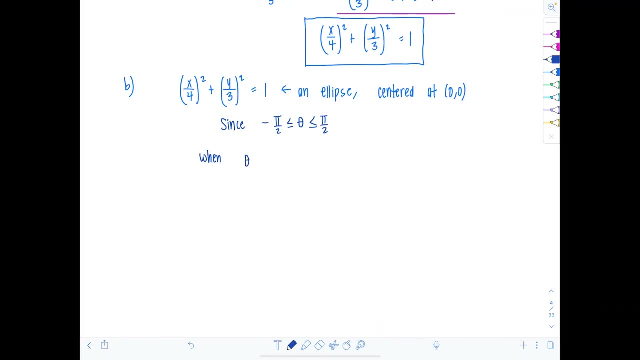 So let's see here: When theta is equal to negative pi over 2, that means x, which is equal to 4, cosine theta would be 0. And y, which is equal to 3, sine theta would be negative 3.. 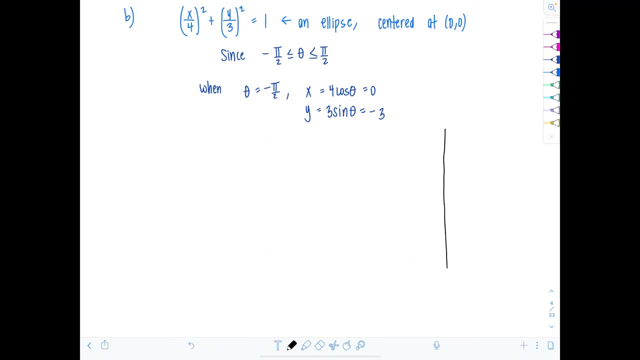 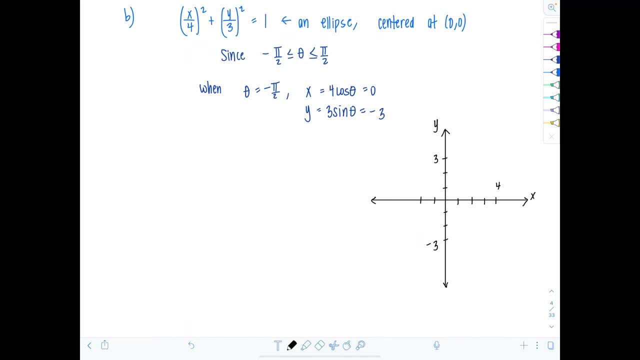 and 4 and negative 4 in the x direction. Okay, and we're starting right here at 0, negative 3 when theta is negative, pi over 2.. Okay, Now what about when theta is 0?? So when theta is 0, x is going to be 4 cosine of 0,, which is 4.. 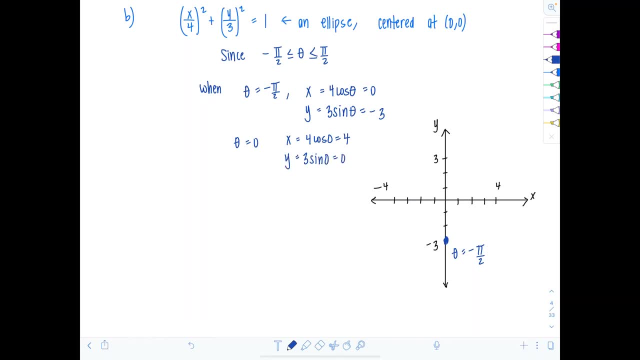 And y is going to be 3 times sine of 0, which is 0. So we'll be right here. So here's this portion. And then when theta equals positive pi over 2, then I'm sure you can figure out: x is going to be 0 and y is going to be 3.. 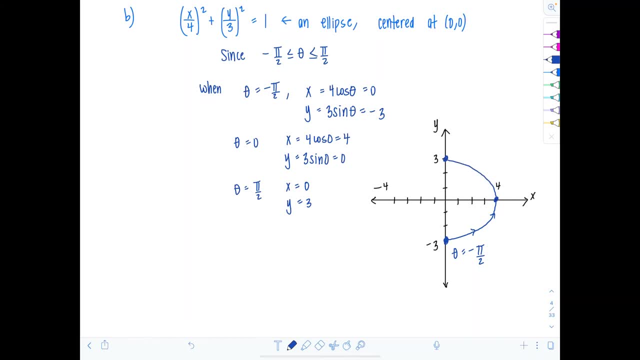 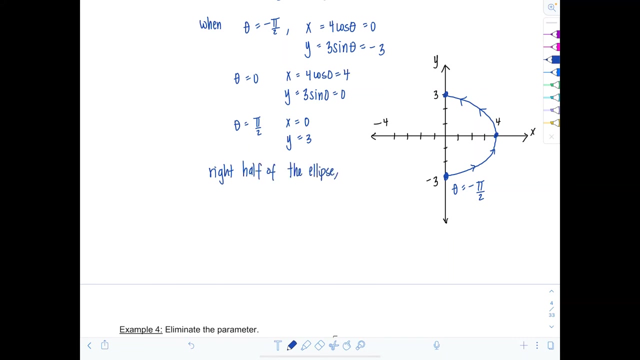 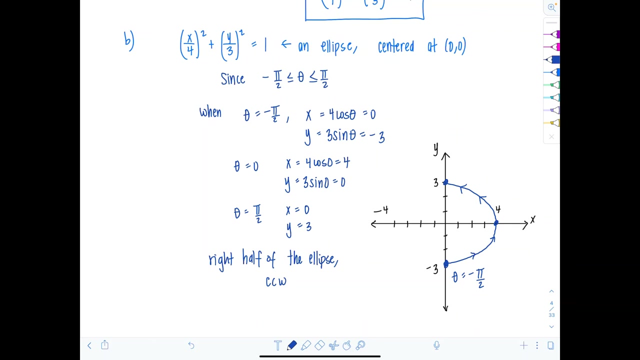 Bada bing, bada boom. So what gets traced out? Only the right half of the ellipse And it gets traced out counterclockwise. So if you'll notice here that corresponds perfectly to the limits on theta being between negative pi over 2 and pi over 2, right. 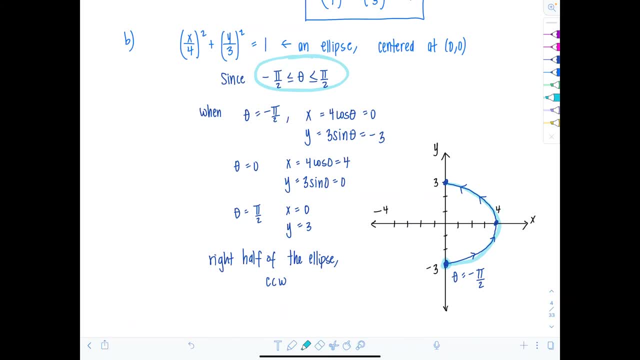 Negative pi over 2 is here up until positive pi over 2.. And if x is equal to cosine theta and y is equal to sine theta and your parameter is increasing, your curve gets traced out counterclockwise. So keep that in mind because later in Calc 3, you're going to have to parametrize curves. 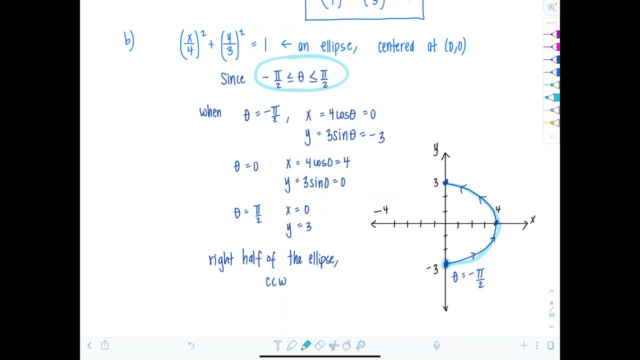 Very nice. Okay, we're just going to practice more eliminating the parameter, but not necessarily graphing. Okay. so here we have: x equals natural log of t And y equals radical t. They also told us ps t is greater than or equal to 1.. 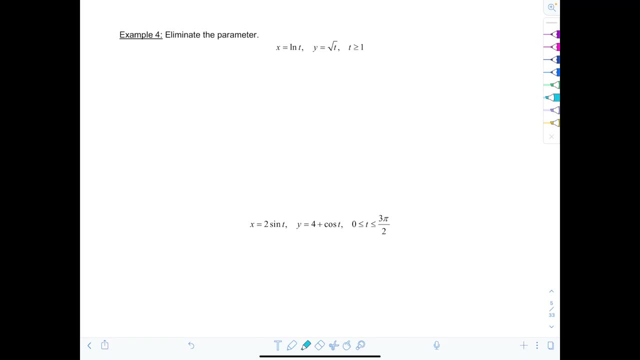 All right, that's probably to make sure everything was going to be nice and well-defined, And I'm just going to go for substitution. Now let's see here which of the two equations would it be easier to solve for t in? Well, if I use x equals natural log of t, I'm going to have t equals e to the x. 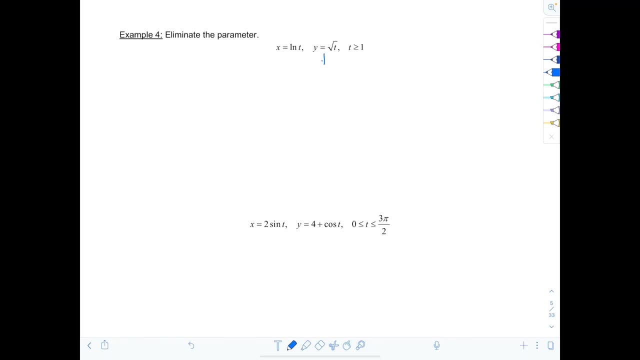 I don't know how nice that's going to be. Let me just go to equation 2 right here, Because I could just say t is equal to y squared. Okay, and then from there, if I replace that into the first equation, 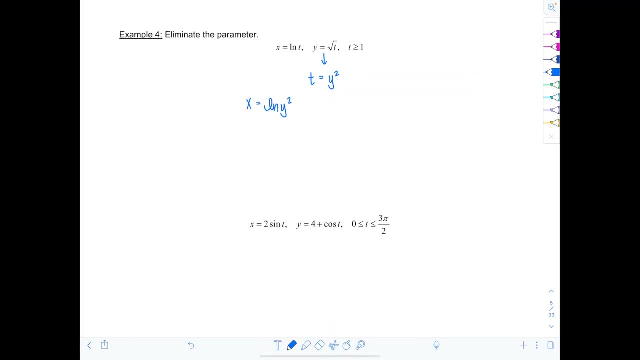 then I get x equals natural log of y squared, which you could leave alone like that, Or I would be allowed to move the exponent to the front. I could write x equals 2 natural log of y, Because they did tell me that. 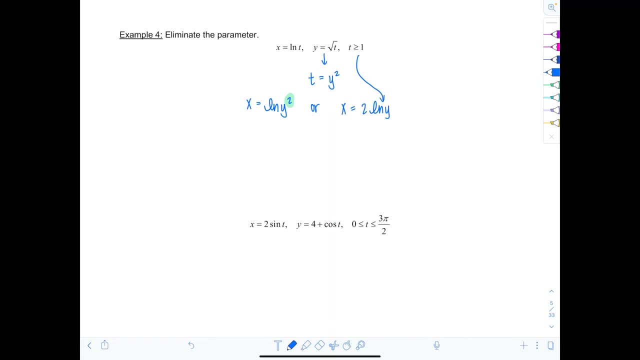 That t is greater than or equal to 1.. So then, that means for sure, since t is equal to y squared, or y equals rad t, t is not going to be negative, y is not going to be negative, And so then we're fine to go ahead and use that property. 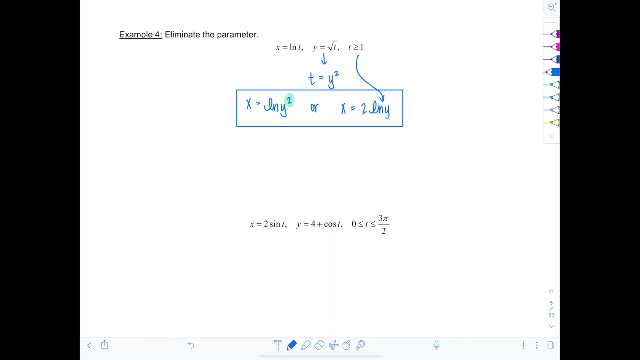 Either one's acceptable. Now, what if I had done it the other way, that I kind of talked myself out of? Would it have been so bad? Let's see If I rewrote it Using the first equation, that e to the x is equal to t. 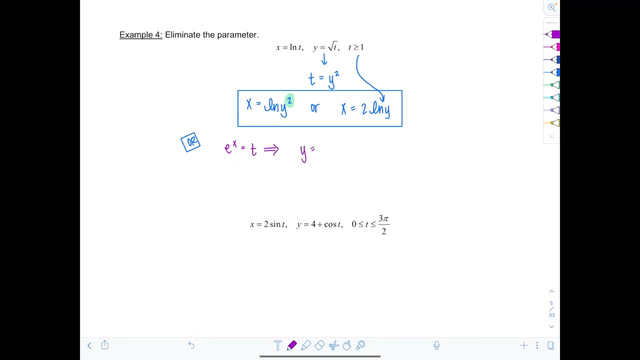 If I substitute that into the second equation, then I get y equals the square root of e to the x, So e to the x raised to the 1 half right. Same thing. And then I end up with y equals e to the x over 2.. 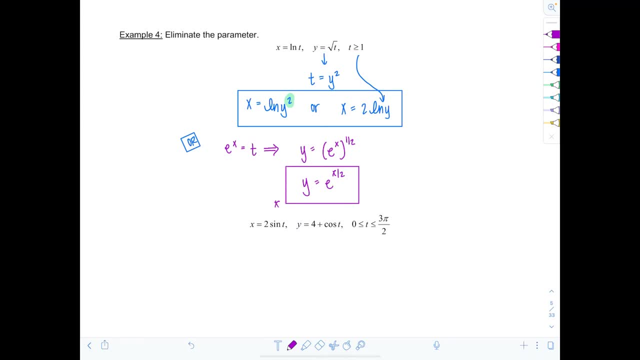 Hmm, Well, they don't look the same, because this gives me a function of x, And the first way It gave us a function of y. Which one do you want? It just depends. What are you going to use these equations for? 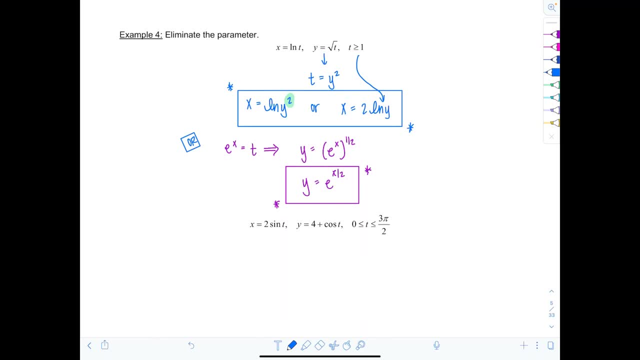 Okay, So it's good to know both ways. I think they were actually both equally tricky, So whatever. Next example: x equals 2 sine t, y equals 4 plus cosine t, And t is bounded between 0 and 3 pi over 2.. 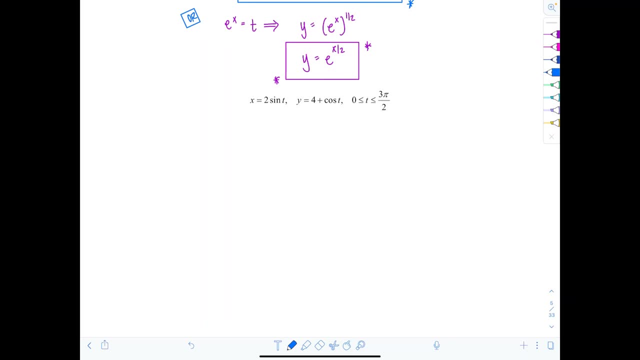 So we're going to use the same technique that I showed you before in the previous example, where we're going to use the Pythagorean identity. In this case we just have to do a little bit a different style of rearranging. So, since x equals 2 sine t, 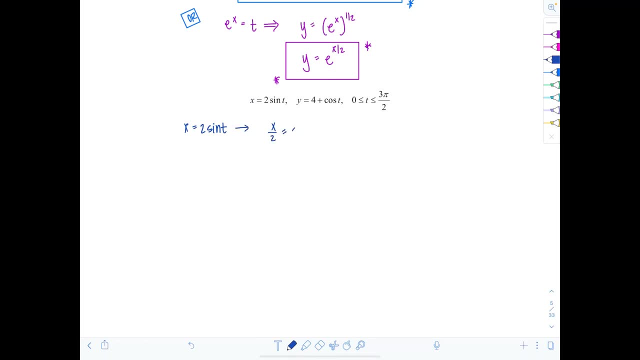 that means x divided by 2 is sine t, Which means x divided by 2 squared is sine squared t. And also, since y equals 4 plus cosine t, then y minus 4 equals cosine t. Okay, So y minus 4 squared equals cosine squared t. 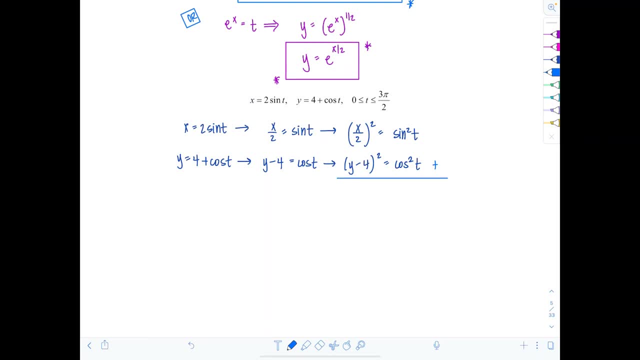 And then we add these together And lo and behold, we have x over 2 squared plus y minus 4 squared is equal to 1.. All right, So this time we have another ellipse. Where's the center, though? Good? 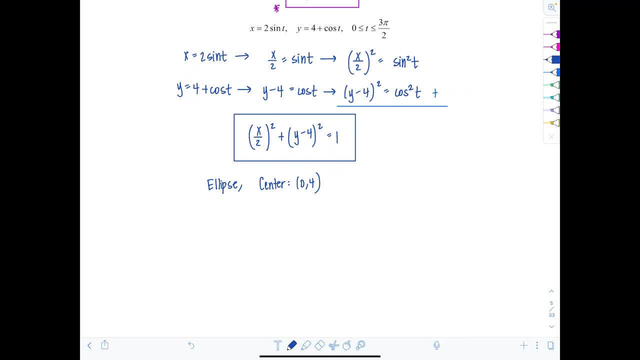 It's at 0,, 4.. And I'll let you play around with it and figure out which portion of the ellipse is traced out and in what direction. So notice, the limits for t are between 0 and 3 pi over 2.. 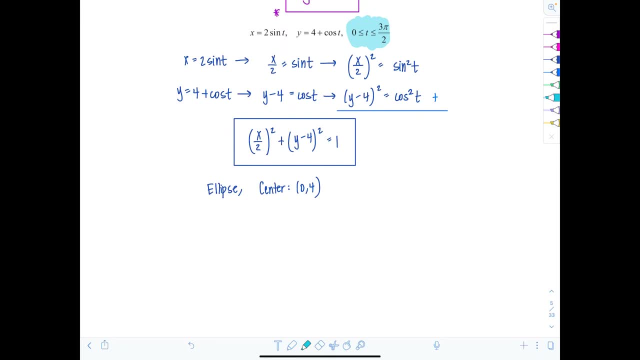 But in this case x is equal to 2 sine t and y is equal to 4 plus cosine t. So play around with it, Plug in. I would say: plug in 0 for t, See where you are. Plug in maybe pi over 2, then pi and 3, pi over 2.. 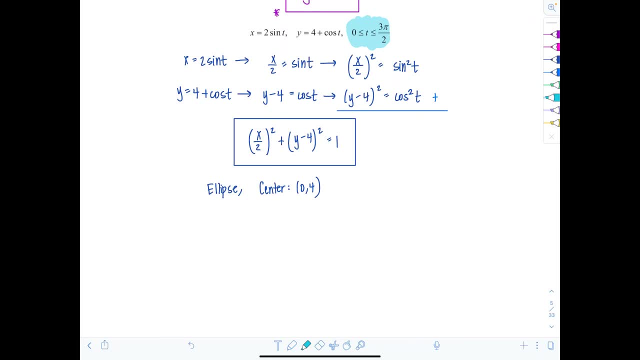 See which part you want, See which portion of the ellipse is traced out and the direction. You can't just do the starting point and the stopping point. Okay, Comment down below what you get. And last example: Couldn't finish this off without some good old hyperbolics, right? 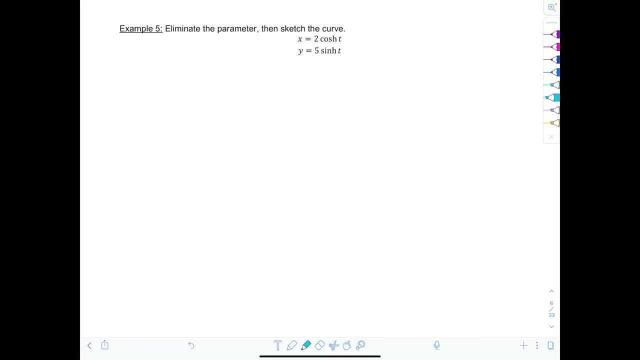 So eliminate the parameter, then sketch the curve. So we have x equals 2 cos t and y equals 5 sin t. We have to use one of the identities That holds for hyperbolics, Do you remember them? So we have cosh squared t minus sinh squared t equals 1.. 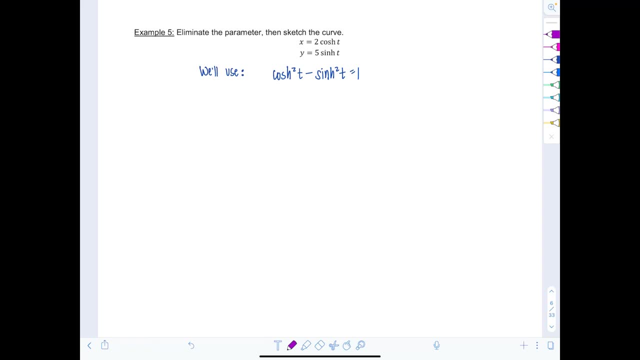 Ooh, oh, my, Okay. So we're going to start off very similar. I'm going to kind of run through the beginning steps a little more quickly. So we'll have x divided by 2 squared, That equals cosh squared t. 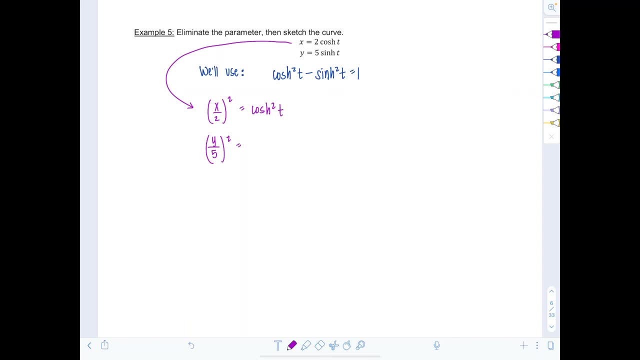 And then I have y, divided by 5 squared, That equals sinh squared t. And remember, for the hyperbolics, this identity involves subtraction. And so now we're left with the equation: x divided by 2 squared, minus y, divided by 5 squared, equals 1.. 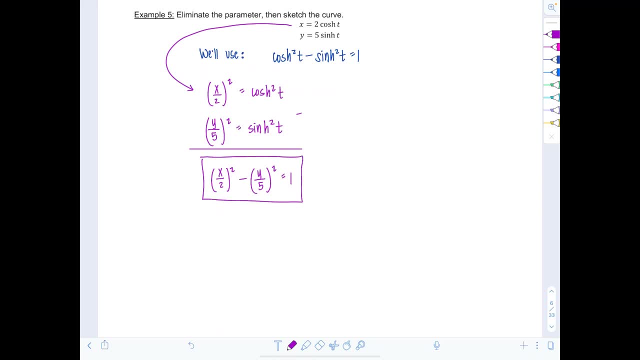 Do you recognize this? Oh my goodness, Maybe if I rewrote it as: x, squared over 2, squared Minus Minus y squared over 5, squared equals 1.. That probably didn't do anything for you. This is a hyperbola. 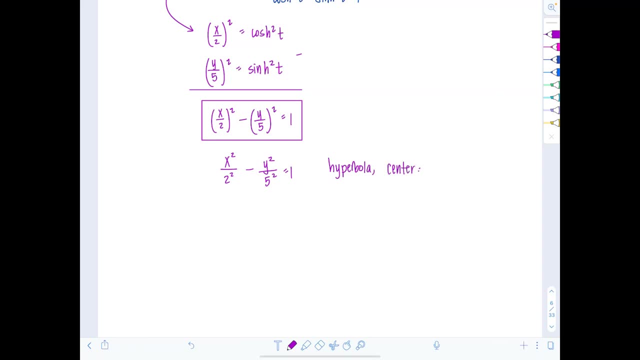 Okay, The center is at 0, 0.. And we're not going to find the foci or anything like that. But I'll just draw quickly the asymptotes. I know it's opening along the x-axis right, Because x squared is positive here. 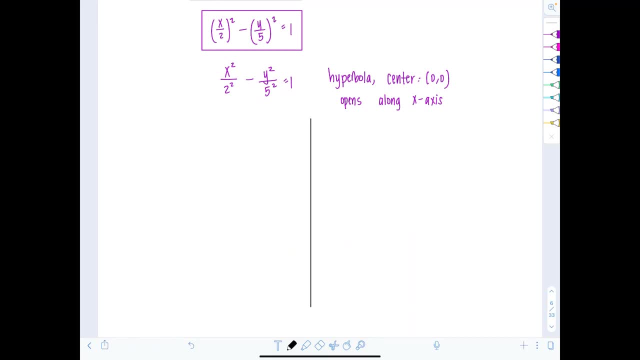 And either, depending on who your instructor is, you're going to study conics shortly after or you've just reviewed them. I'll link a video here if you need a review on hyperbolas. Okay, So the center is at 0, 0.. 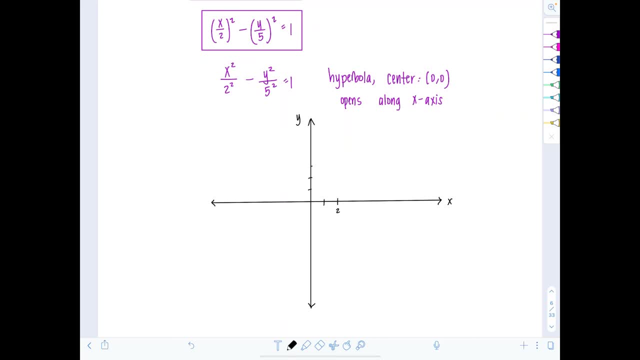